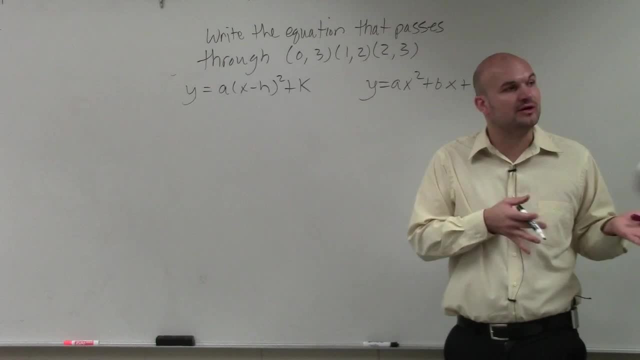 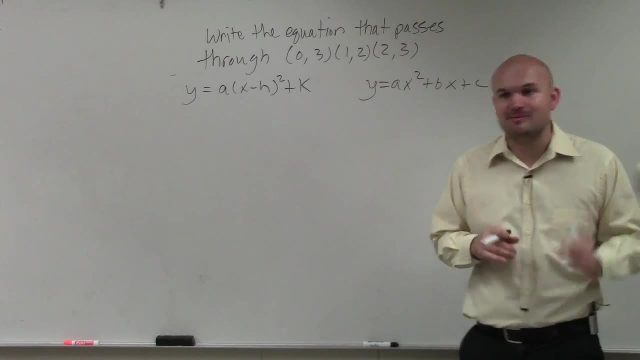 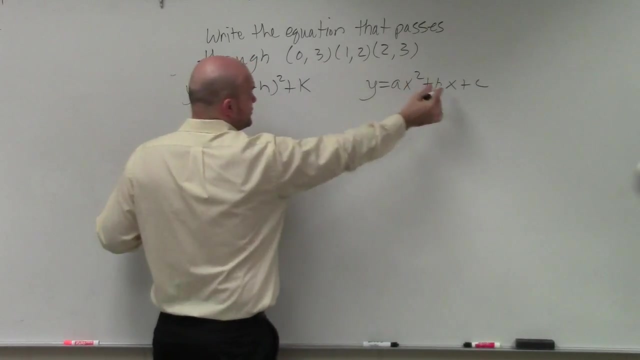 call a system of equations. If you guys remember, in unit one we learned how to solve using substitution and elimination. We're going to come up to the same thing, So let me just show you what I mean Basically. what I'm going to do is I'm going to plug in each of these three points into this. 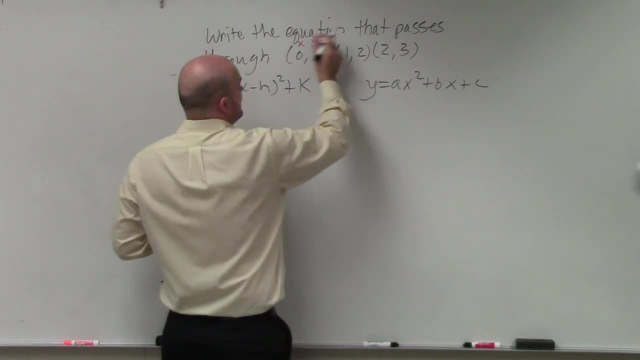 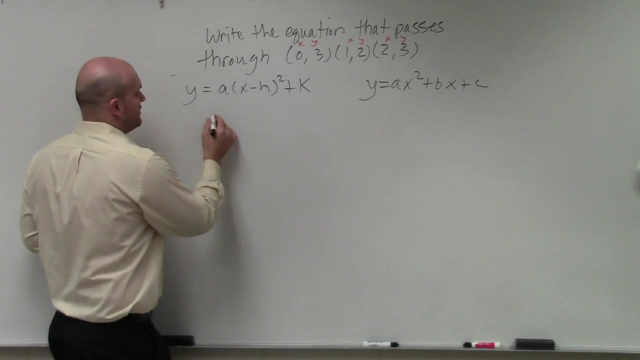 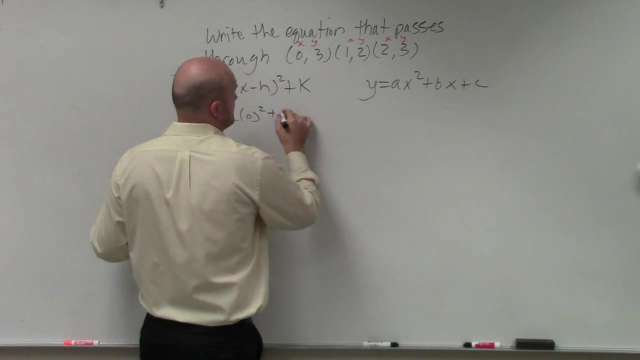 equation for x and y. These all represent x and y. Everybody follows me Okay. So if I plug them all for x and y, I have 3 equals a times 0 squared plus b times 0 plus c Over here. 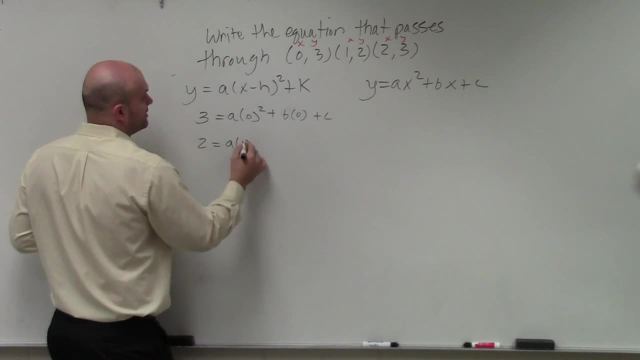 next one, I have 2 equals a times 1 squared plus b times 1 plus c. And the last one, I end up having 3 equals a times 2 squared plus b times 2 plus c. Does everybody see what I did? I'm not using 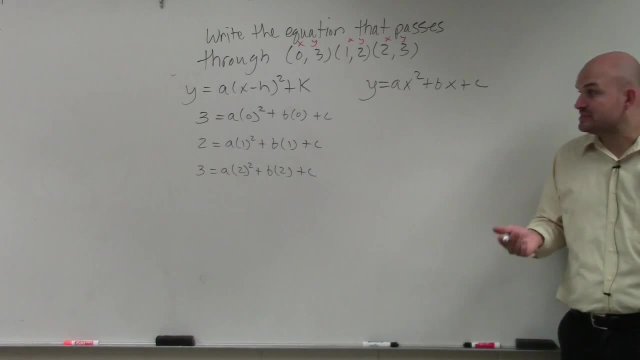 vertex form. in this one I'm using standard form, And the reason why I'm using standard form is now let's go and simplify what this is. Well, this all goes to 0, right, So you could say c is 0,. 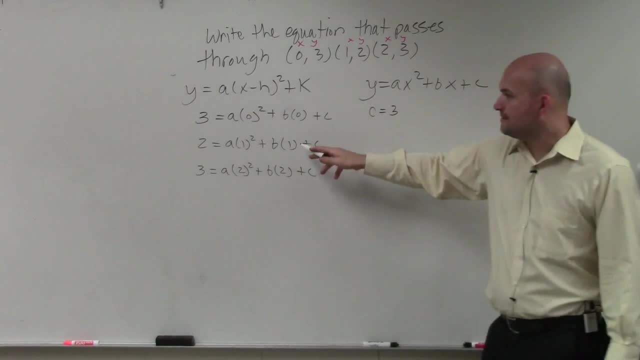 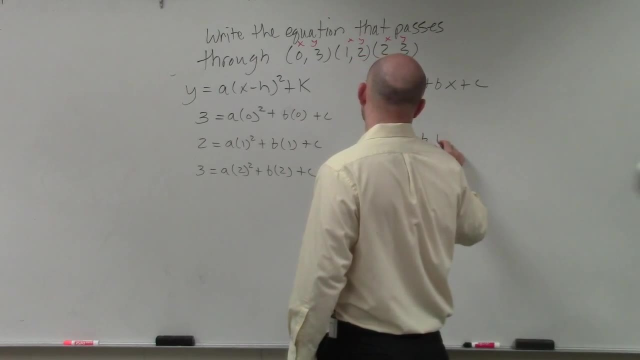 c equals 3.. Here this goes ahead and simplifies to the equation: 2 equals a plus b plus c. And then this one simplifies to: 3 equals 4a plus 2b plus c. Now in this class we did not cover how to solve. 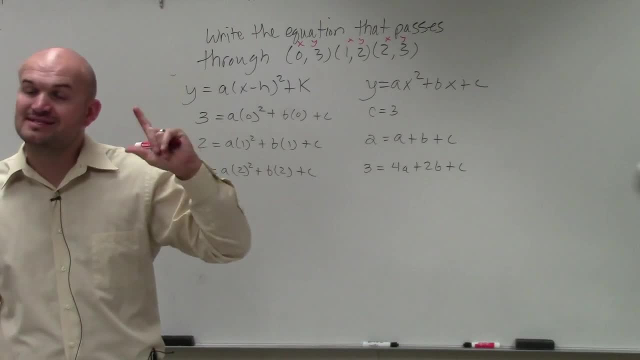 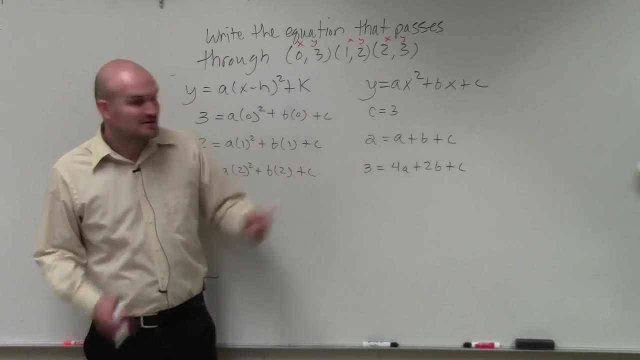 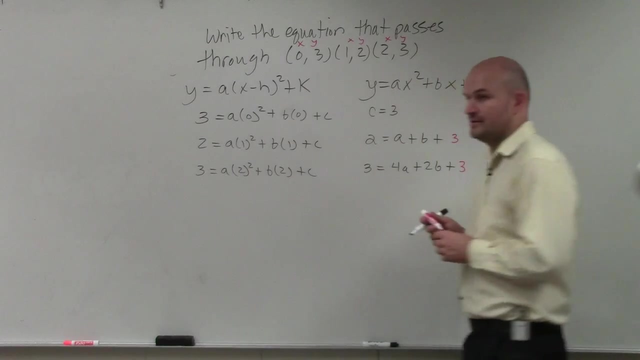 a system of equations with three variables. However, what's nice about this is we know what the value of c is. right, You guys agree with me. So guess what I can plug in? I can replace c with 3.. So if I replace 3, let's just use that 3.. 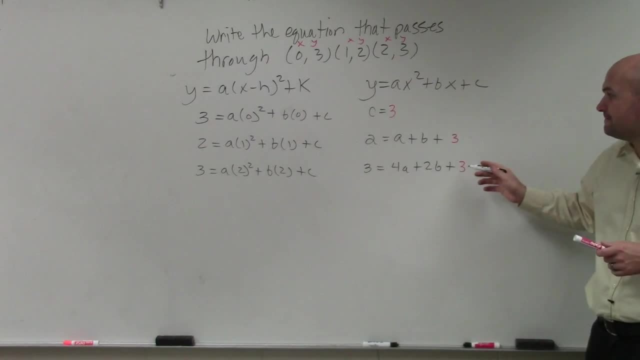 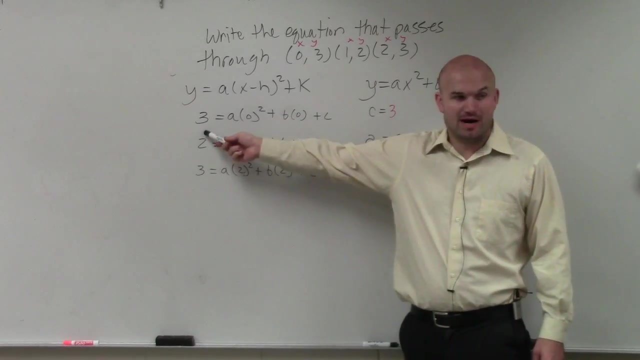 If c equals 3,, I can replace c with 3, and then I have a system of equations. So what I'm going to do? yes, How do you know that c equals 3?? Well, because when you plug in the point 3 and 0, 0, in for the x's, 3, in for the y, 0, 0, c, c equals 3.. 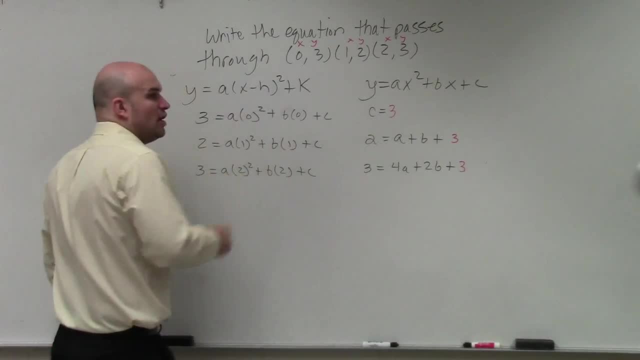 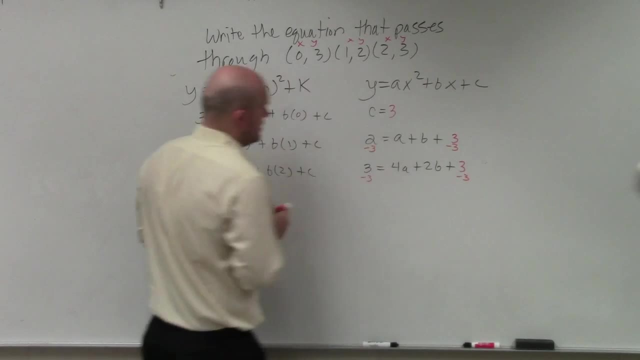 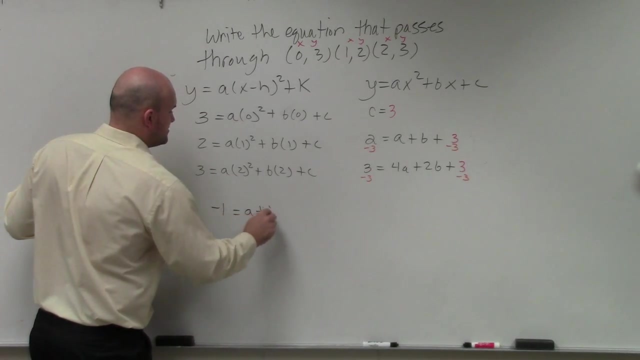 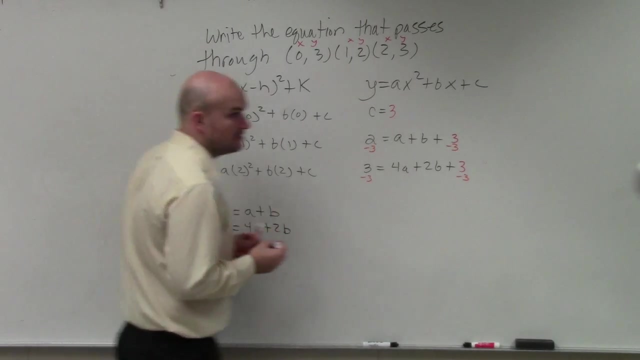 Make sense. Those all go to 0. So now, if I go ahead and solve each of those, I get my variables on the same side. I get this equation: Negative: 1 equals a plus b. divided by 0 equals 4a plus 2b. 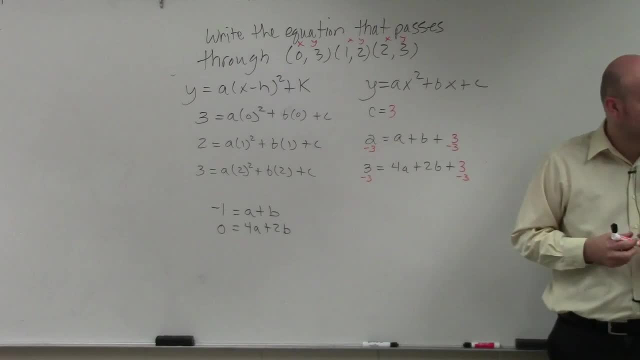 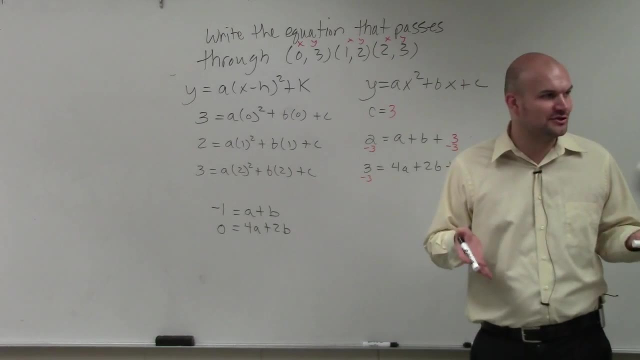 Do you guys remember when we did systems of equations like this? Now, the reason why I'm going to give this problem is, if you guys remember, on your first unit one test, did I actually assess that you could do elimination or substitution? No, it was like all these stupid word problems, right? 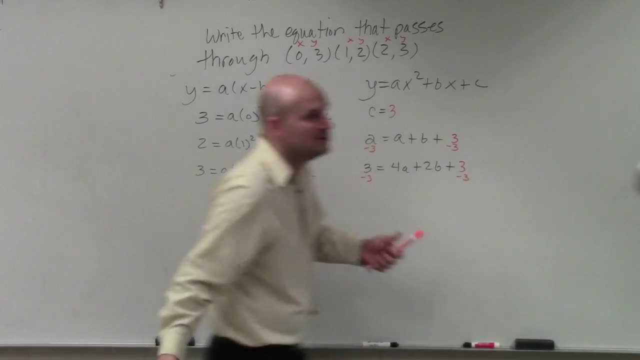 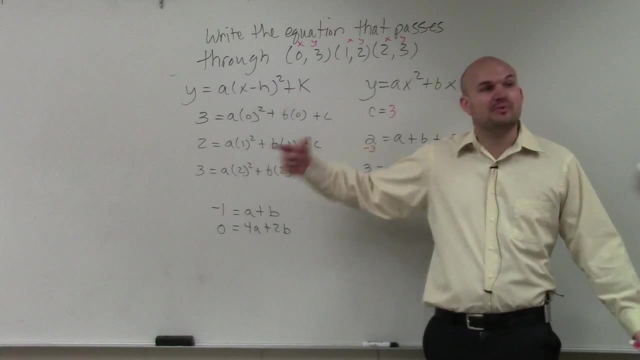 Well, guess what? Here's an opportunity for you to show me that you can solve using substitution or elimination. So remember, you could either solve for a or b and plug it into the other equation. However, in this example, I would like to use elimination. 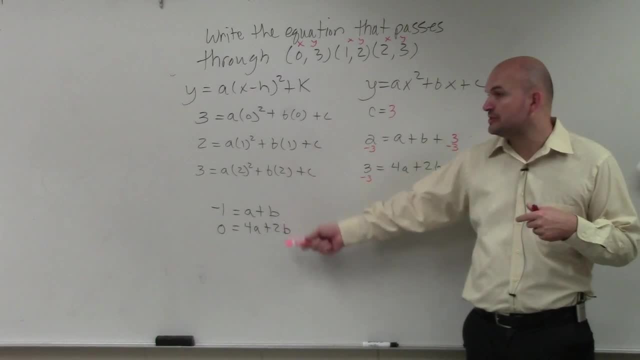 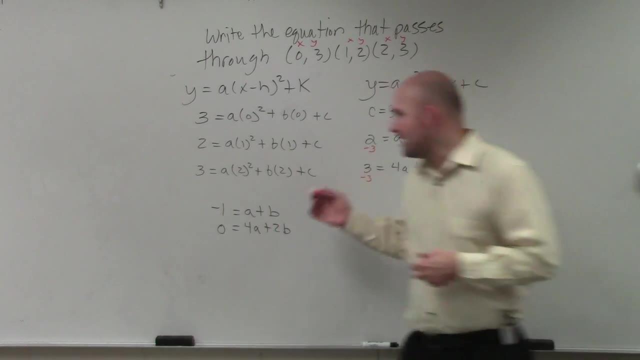 My preference would be to eliminate the b. Remember, when you're doing elimination, you want to get the variable having the same coefficient. I like to always do one positive, one negative, So therefore I'm going to multiply the top equation by a negative 2.. 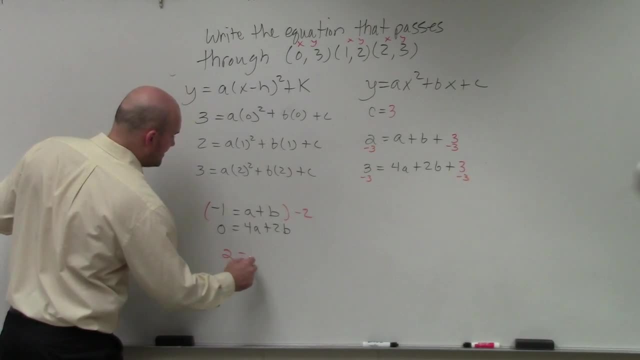 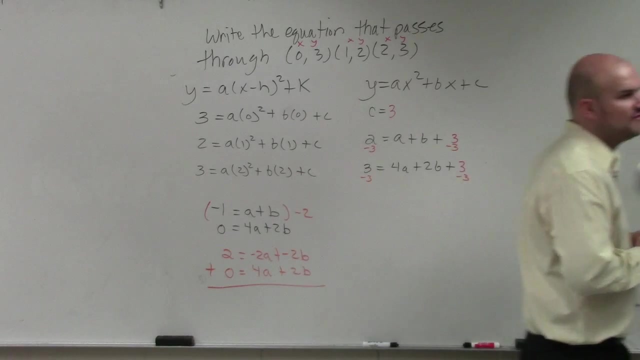 By doing that I now obtain Positive 2 equals negative 2a plus negative 2b. all over 0 equals 4a plus 2b. Do you guys see that b both has the same coefficients, One's positive, one's negative. 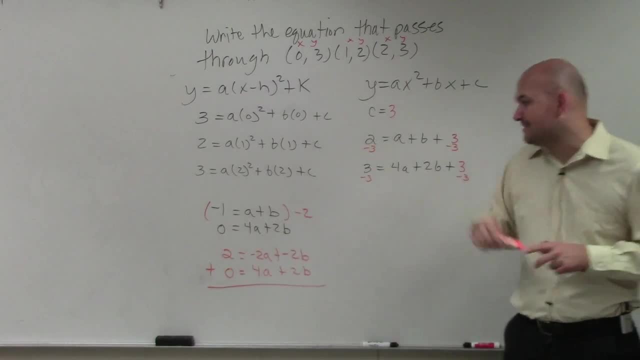 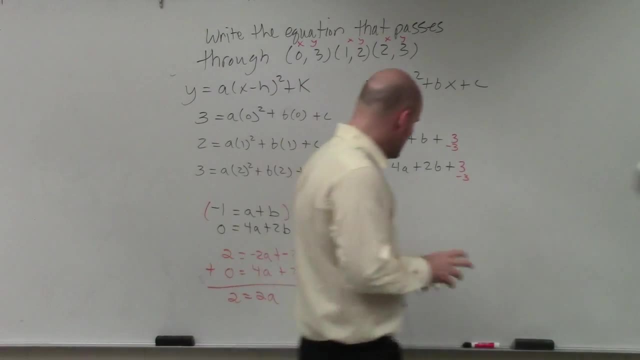 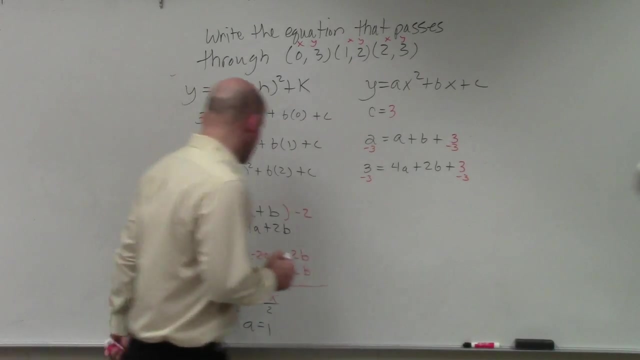 You guys see that? Yes, Now I add them vertically and I get 2 equals 2a. So now to find a, I simply just divide by 2.. a equals 1.. Then, once I know what a is, I can plug 1 back. 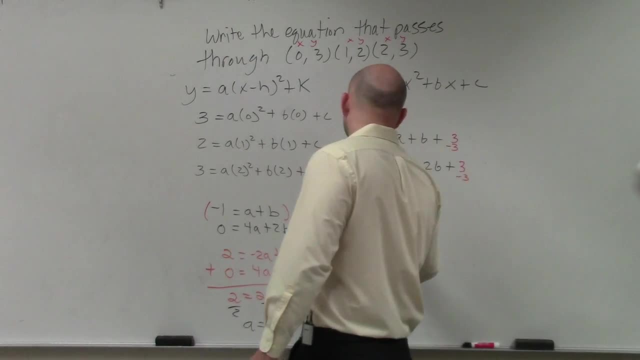 into one of my equations to solve for b. So I'll go to: negative 1 equals a plus b. Negative 1 equals a plus b, Subtract 1, subtract 1.. Negative 2 equals b. So now, ladies and gentlemen, I know,